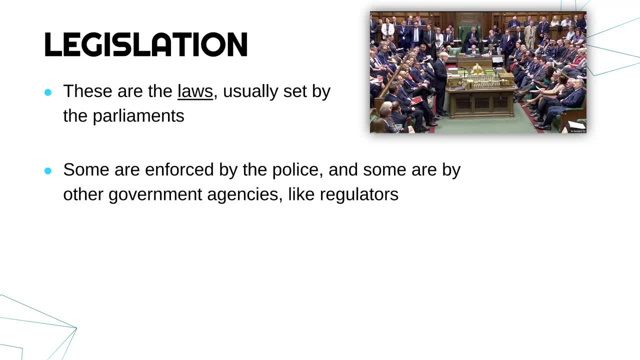 laws as being only enforced by the police, which many laws are. but some laws are enforced by other government agencies, such as regulators, and this law, the Data Protection Act, is an example of one of those which isn't the police don't get involved in. it'll be regulators, and for most laws we're. 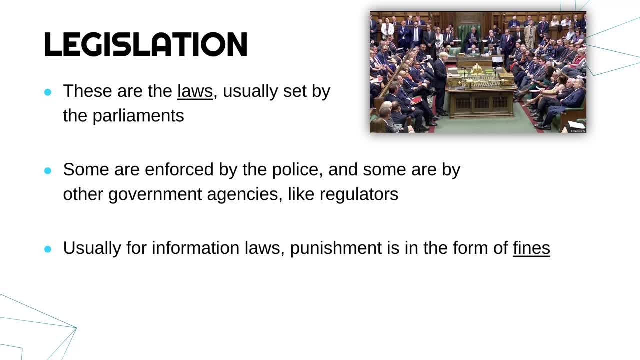 thinking about in IT and for this law, the Data Protection Act, punishment is in the form of fines. people don't get arrested and dragged into prison for breaking these laws, but they can get very, very large fines. and it's not always the police issue these, it can be other agencies. Okay, so one of the 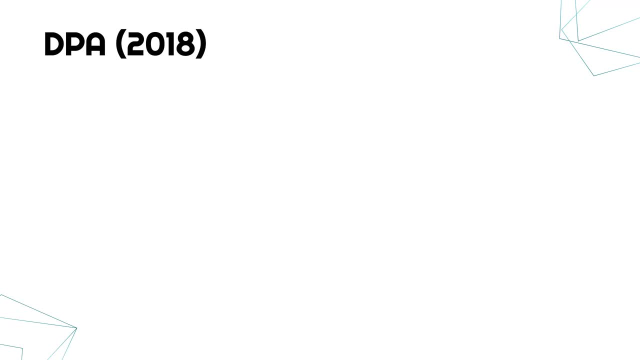 laws which can produce huge fines is the Data Protection Act, often shortened to DPA. So this law, the most recent version, came out in 2018. there was a version which was from 1998, but it's now been updated. This law works alongside the UK's version of a law called GDPR, which originated 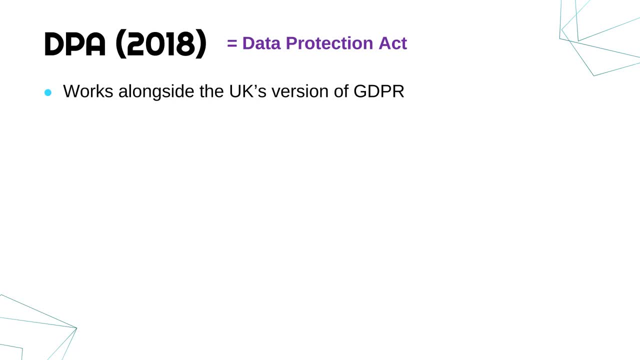 from the European Union, and the UK effectively adopted this European Union law. although, despite it's leaving the EU, we still have it and it works alongside this other UK only law called the Data Protection Act. So the DPA only applies if you are collecting information about people for an 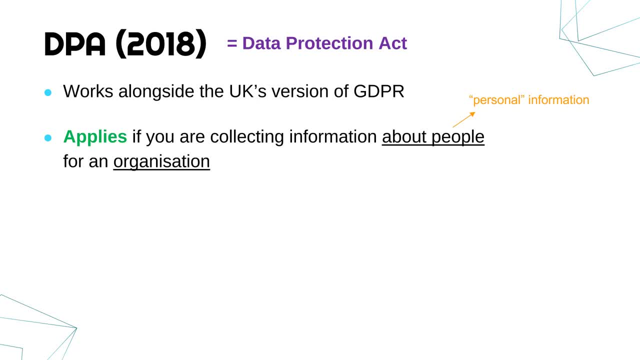 organisation, and so, because it's about people, we're talking about personal information. Now, interestingly, this law doesn't apply if you're collecting information for your personal reasons, you are able to stand on a high street and film people, and that's perfectly fine. but if you're 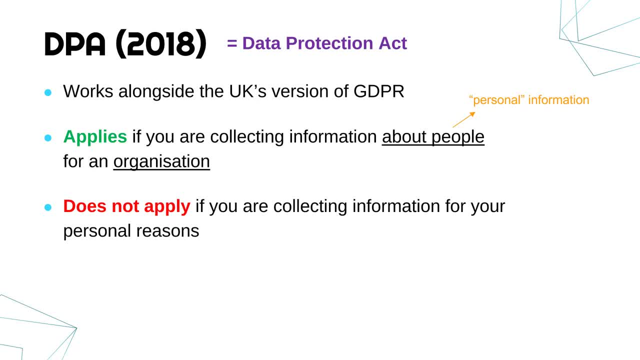 doing it for an organisation, it then comes under this law. So a slightly weird thing here, and it's all about organisations. Now, a couple of key terms which are useful to mention when you're talking about this law are, first of all, data controllers, A data 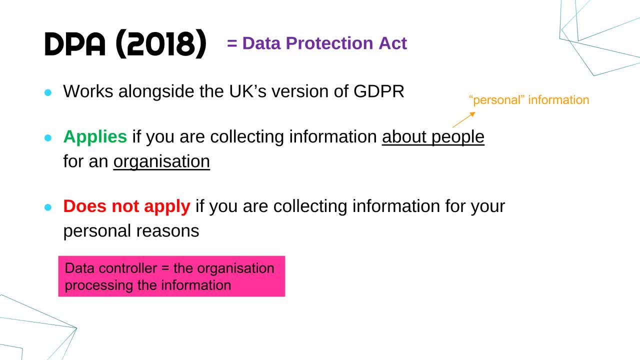 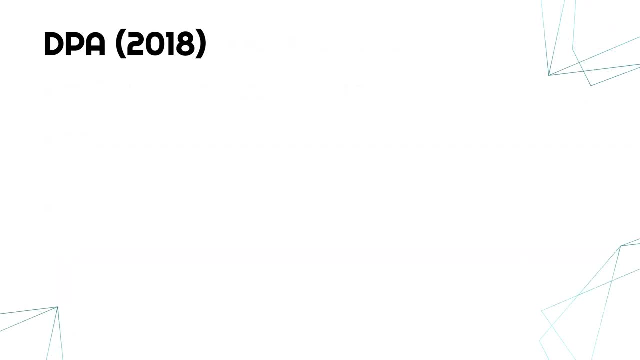 controller is the organisation processing this information and the data subject is the person who the information is being collected or processed about. So, controller, organisation, subject: the individual person. And this piece of legislation requires certain things which data controllers have to do. So a big one which affects all of us every time we go on a 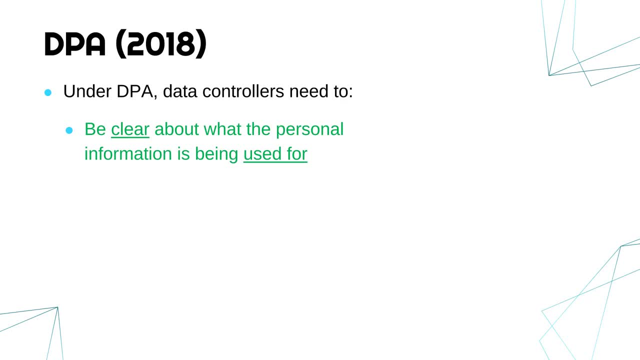 website is. the controllers need to be really clear about what personal information they're collecting and what it is being used for. It's why you get loads of messages when you go onto a new website wanting to accept certain policies. This is the website trying to be clear about what the data is. 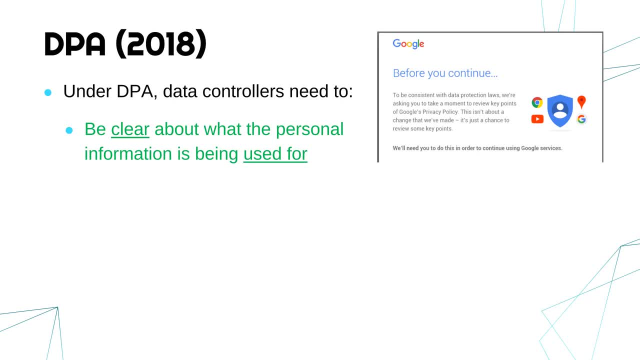 being used for. Whether you read it or not, is it's kind of up to you. The controller also should only be keeping the personal information when it is needed. The second it becomes unnecessary, it should get deleted permanently. They also need to, under the law, provide information security. The law doesn't say specifically what this needs to be or how much they need to spend or what they need to do. but if there was a cyber attack and they didn't have security in place, that is when the fines can really kick in. And security is not only things like antivirus or firewalls or encryption. 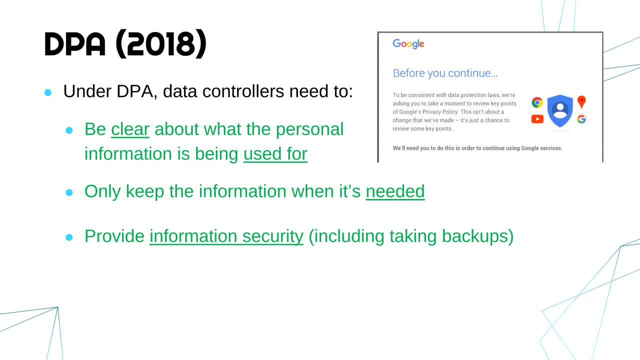 It can also be less, maybe, obvious things like taking backups, which are important as well, And, lastly, the well. it's not not the only thing, but the last main thing I want to mention is controllers also need to make sure the information is kept up to date and is kept accurate. So that's why, again, often organizations get in touch with 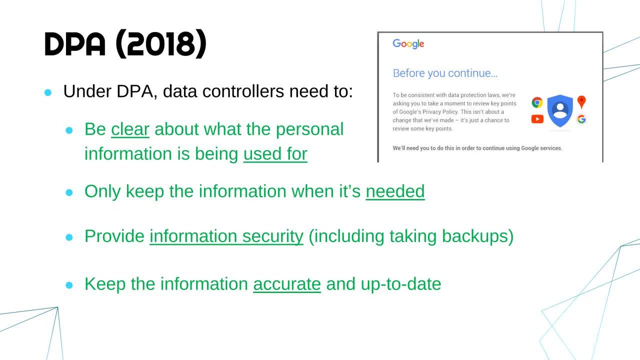 you, asking you to update your address, asking you to update your number. That's partly for their own purposes, but also partly to follow this law. So if organizations don't do any of these four things, then again they could get fined, and that could be millions of pounds in some cases. There are also 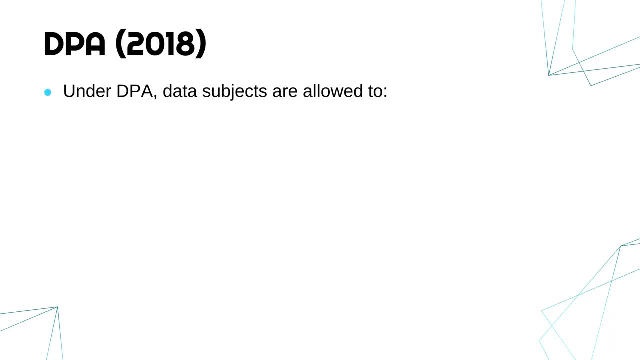 a few things which are specific to data subjects. so, really, rights that all of us individuals have. Well, one right is we are allowed to see what personal data is being stored about us, So we're able to launch what's called a subject access request, sometimes shortened to SAR. This is when 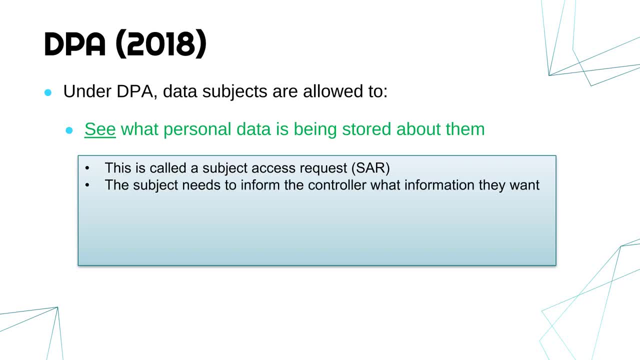 we basically contact, inform the controller about what information you want to see and the organization has to give it to us. They should ask for ID to make sure we're not just requesting some random person's information. So we might provide our passport or something like that, and the controller has to provide this information within a month or explain why they. 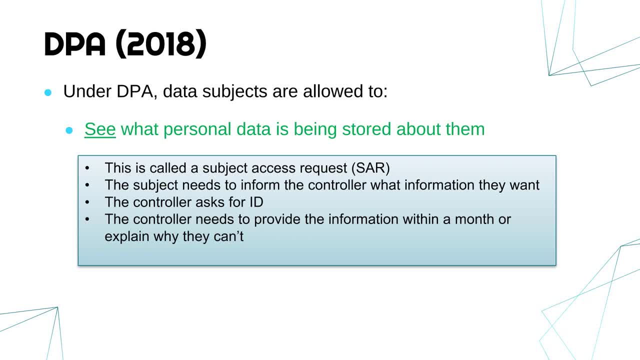 can't So. maybe they can't because it was deleted already. Maybe they can't because it's going to take a month to to do and they just can't afford to do that. So unless they've got a really, really good reason, They have to provide the information.